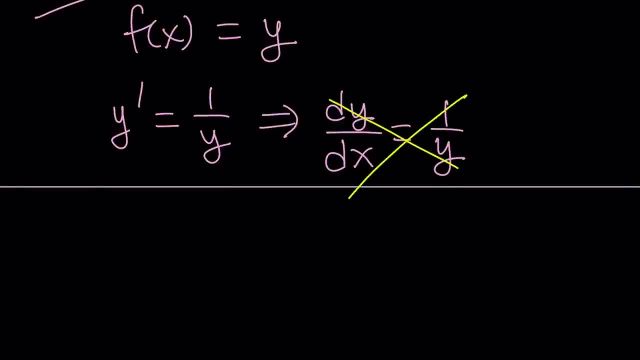 we are going to end up with a separable differential equation. So separable equations are very easy to solve because all you have to do is separate the variables and integrate both sides. So that's the strategy. If you cross, multiply, you get y dy equals 1 dx. 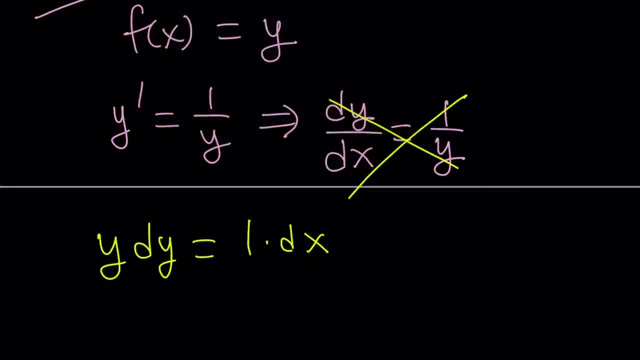 And then, if you go ahead and integrate both sides, then on the left you get y, dy equals 1 dx. And then, if you go ahead and integrate both sides, you're going to get y, the integral of y with respect to y. 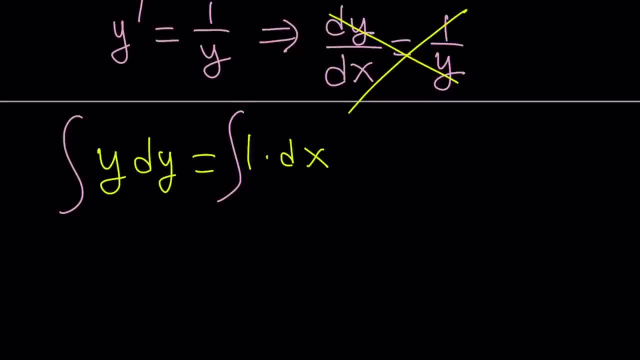 So what's the integral of any power of y, Like y to the n, y to the power, n is y to the power, n plus 1 over n plus 1 plus c. remember As long as n does not equal negative 1, because that's going to cause problems. 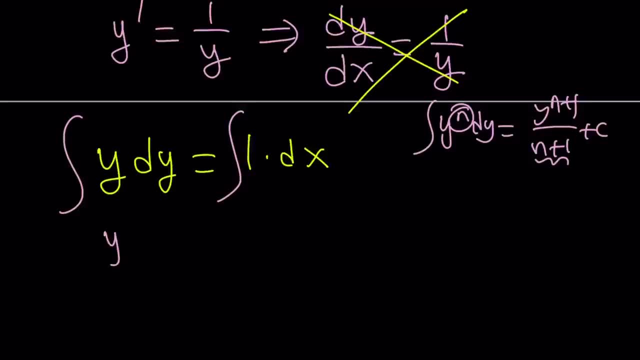 But y is, n is 1 in this case. So we're going to increase the power and divide by that power And I'm going to save the constant for right-hand side, because we only need one constant. So prata equal 1 over x. 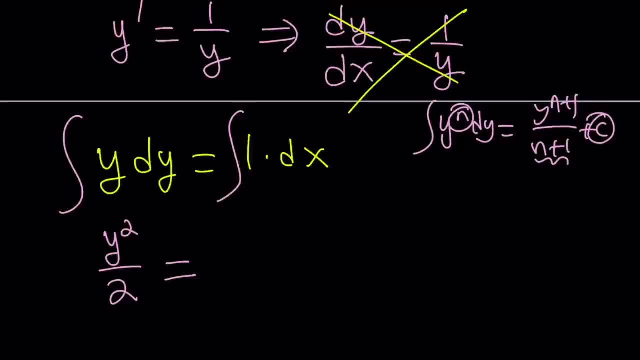 Ok, So I'm going to nose this and turn it in, And if we want the rest of our Jews with us, we're going to minus this hertz, We're going to take this, we're going to move this and this will be 1 over 1 squared. 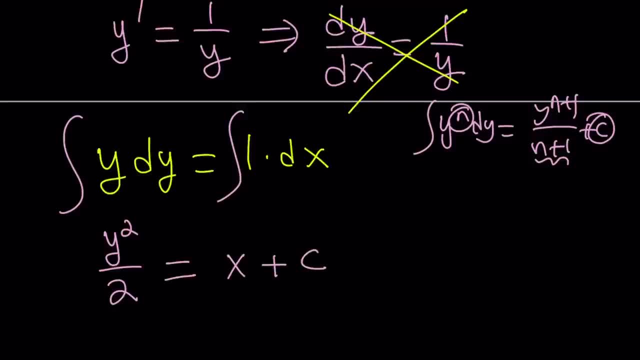 general notice: 0.. So this is the derivative of divided by 1.. So we're already doing thequila here. We should know this whole temperature. Subtitles byнев. Think about it In terms of derivatives Or anti-derivatives. 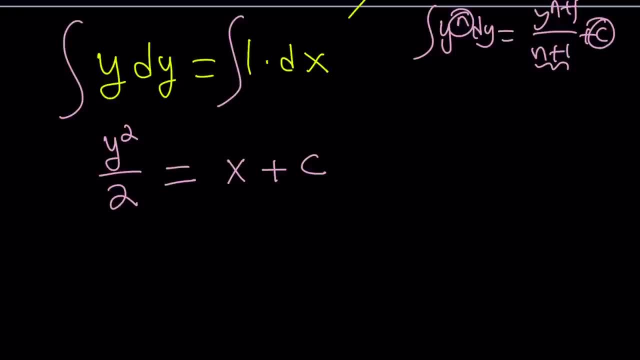 that makes sense. now we're going to go ahead and multiply both sides by 2. that's going to give us y squared equals 2x plus 2c, 2c or not 2c. and then, since c is a constant, 2c is a constant we can. 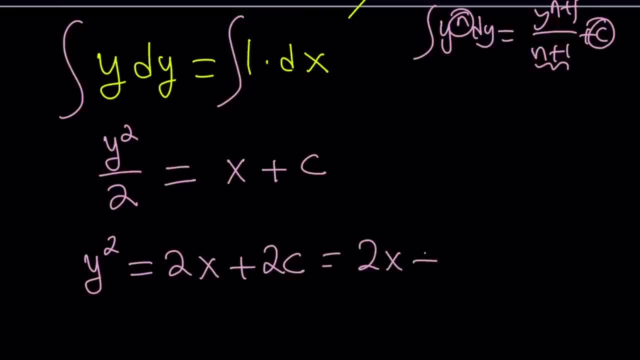 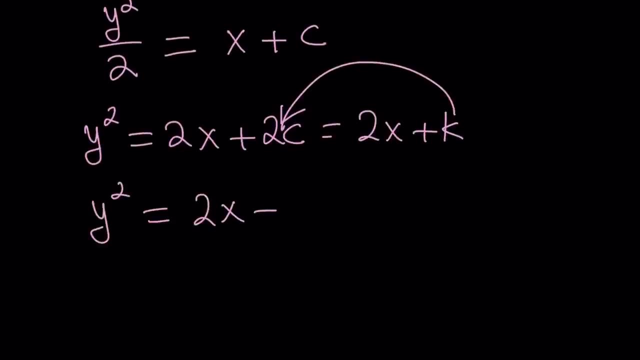 replace it with something like k. k is another constant that represents 2c. okay, so now we got this equation: y squared equals 2x plus k. so that's the function we're looking for, but it's y squared right. so i want to get y and obviously we take the square roots. but there are two solutions that 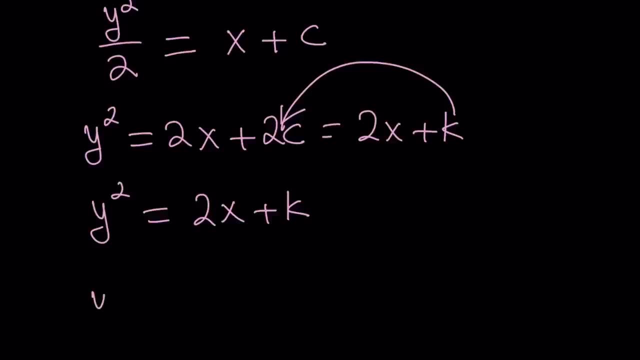 come from absolute values. right, absolutely. so that gives us y equals plus minus, the square root of 2x plus k. so that kind of gives you two solutions. and since the constant is inside, we still have to use the plus minus sign. sometimes, when you have a constant, like you know, you'll be getting solutions. 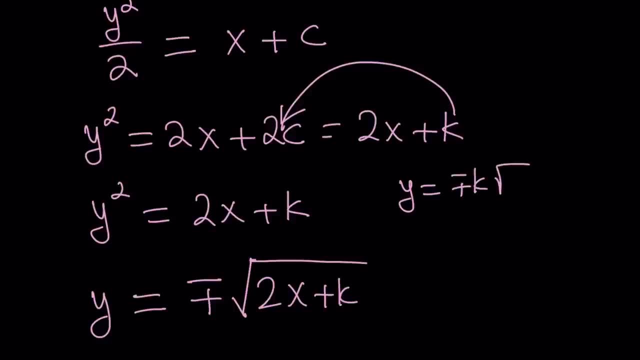 like y equals, you know, plus minus k times something, something thing. In this case you can kind of forget about the plus minus, because k can be positive or negative, so it'll take care of every value Make sense. But we don't have that, so we have to keep. 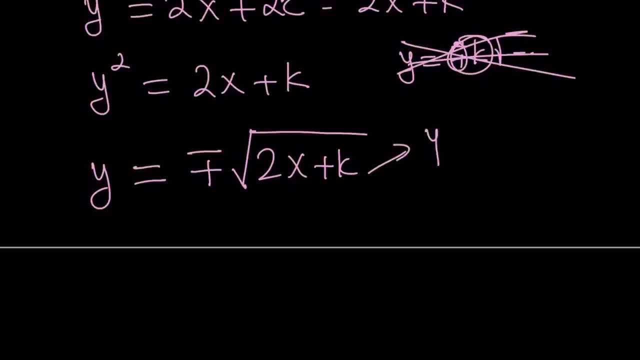 it And we can kind of split it up if you want. y is either square root of 2x plus k or y is square root negative of that. okay, So when I ask you the question what type of function, when differentiated, gives you its reciprocal, the answer would be that: And if k is zero? 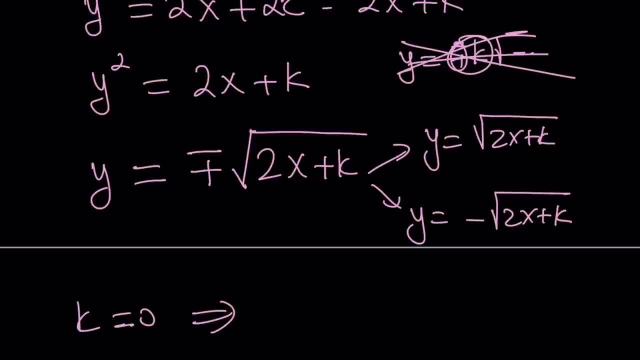 obviously, then you get a special solution And obviously, if we had initial conditions, then you could use them to find the value of k, which would be determined by the initial conditions. And by the initial conditions I mean something like, let's say, if they tell you f of 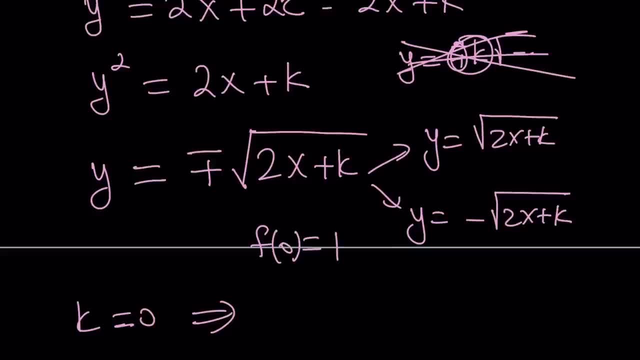 zero is equal to one. okay, Then you would replace x with zero and set it equal to one, And from there you would find the k value Make sense. Okay, We don't have that. but if we did, what you would do is you would say: hey, f of x is equal to the square root of. 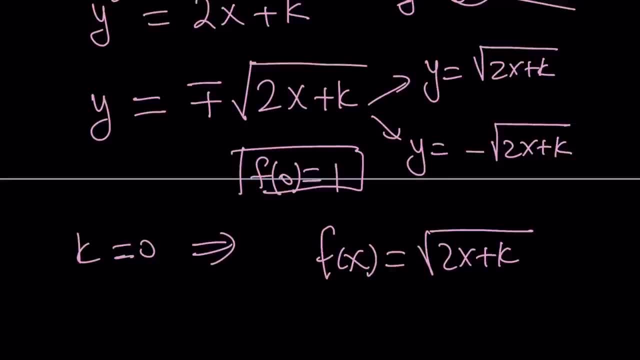 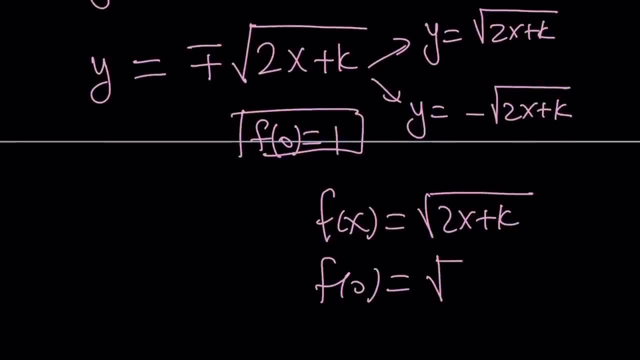 2x plus k. in the first case scenario- And let's just forget about the k- is zero, for now I don't want to confuse you. And now f of zero is going to be the square root of k, And if this is one, 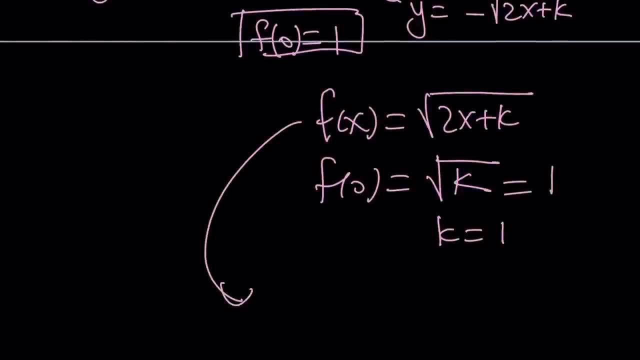 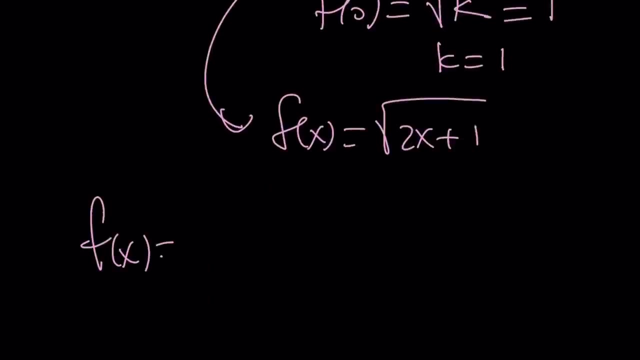 that means k is equal to one, And then plugging it back in would give us f of x equals square root of 2x plus one, And that will be the solution, the particular solution for this initial value. But if you use the second one, f of x equals negative square root of 2x plus. 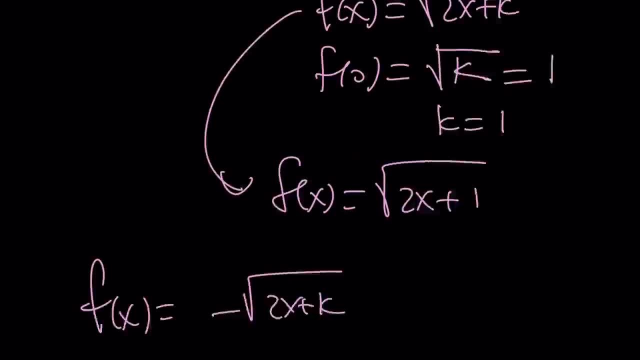 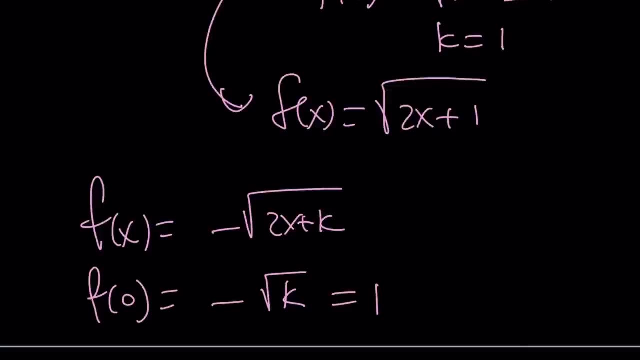 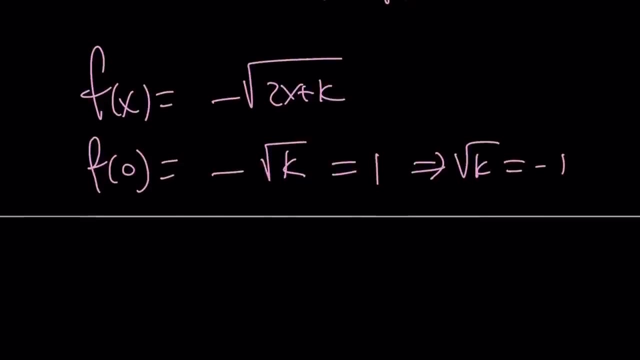 k And if you plugged in zero, f of zero would be negative square root of k, And if this is equal to one, then that would mean the square root of k is negative one. But from here you would not get a real value because there is no real number whose square equals, I mean whose square root. 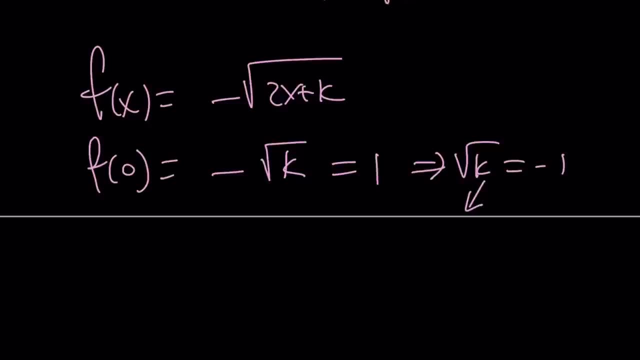 equals negative one. Okay, That would be one again, But this time we would be dealing with a complex number. Make sense, If you think. in the complex sense one has two square roots. That's why one to the power, one half, is equal to negative one. in one of the problems that we recently did. It's a little bit. 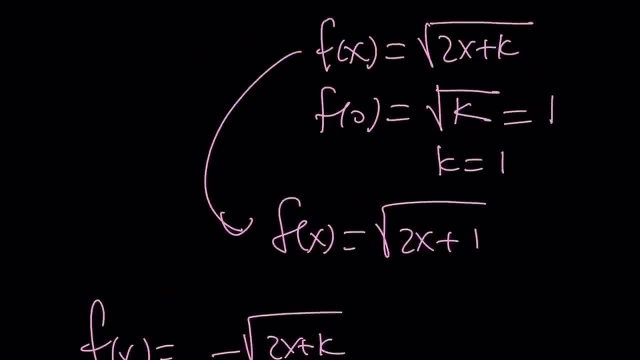 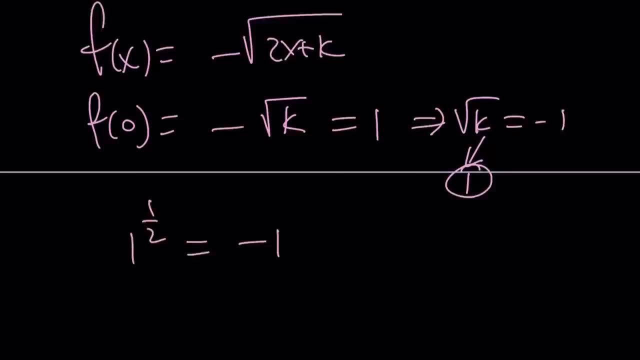 of abusive notation, but that's okay. Now, so in the second one we kind of get an interesting scenario, But that's basically what it is with an initial value scenario. I just wanted to give you that. So let's go ahead and take a look at the second method. 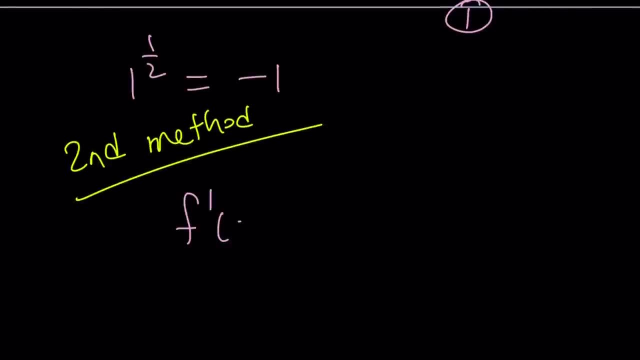 With the second method. let me rewrite the problem. f prime is equal to one over f, So hopefully you're convinced that this radical function will satisfy this and you can always test it out and we'll do that. So now we have this scenario. Let's multiply f of x times f. 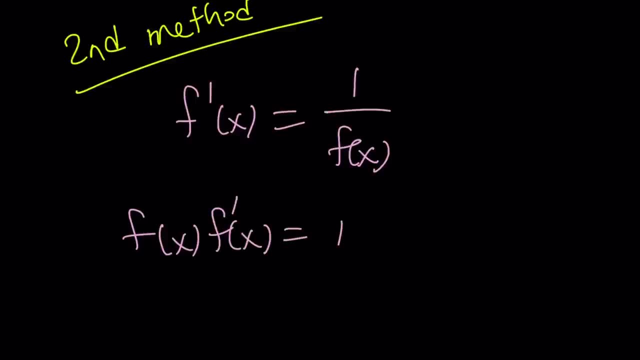 prime of x equals one. Now this kind of tells me why don't we multiply both sides of the integral? So I want to multiply both sides by, and let me kind of space it out a little bit like this: I want to multiply both sides by dx, And the motivation behind it is: I want to integrate this. 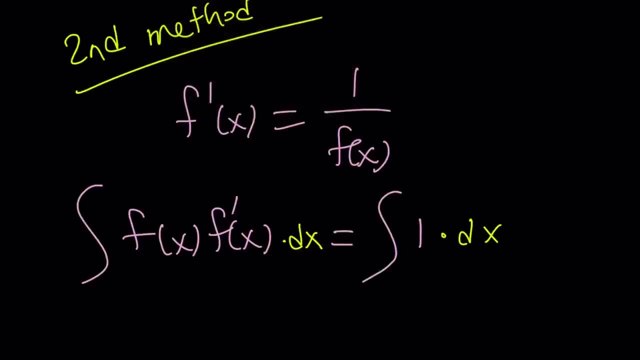 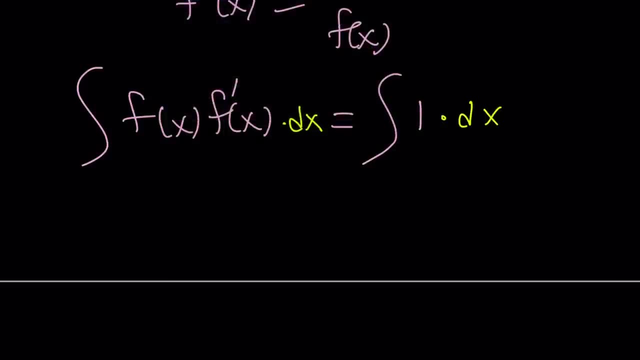 thing. So let's go ahead and do it. If you integrate both sides, you get this integral equals. that integral Right hand side is easy, but left hand side, let's use substitution. I know we're kind of stretching this, but if you call this u, this will be du right. So we have the integral of. 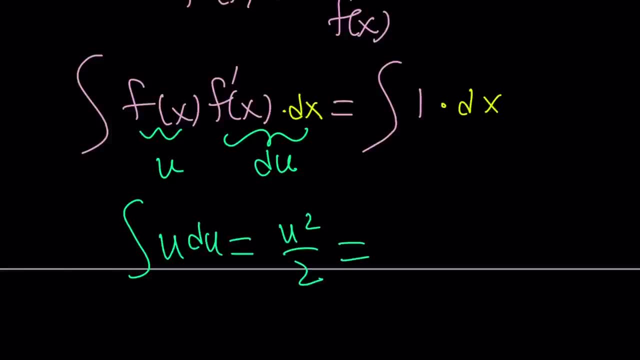 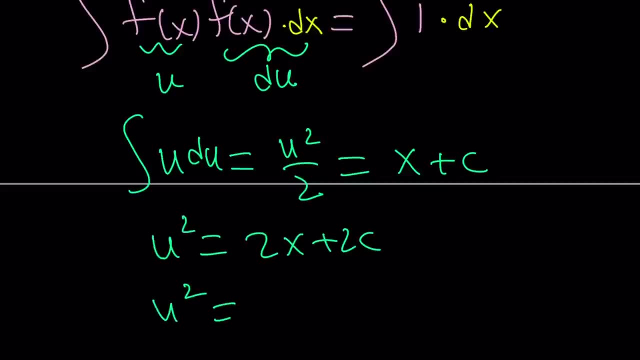 u du, which is u squared over two, and that equals x plus c, And if you multiply by two, you get 2x plus 2c, which can be written as 2x plus k again, k being a constant, And then u is. 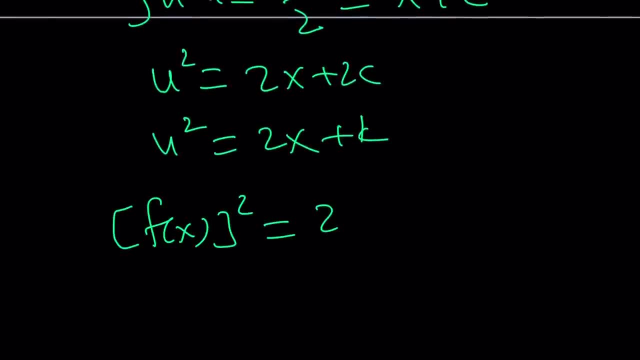 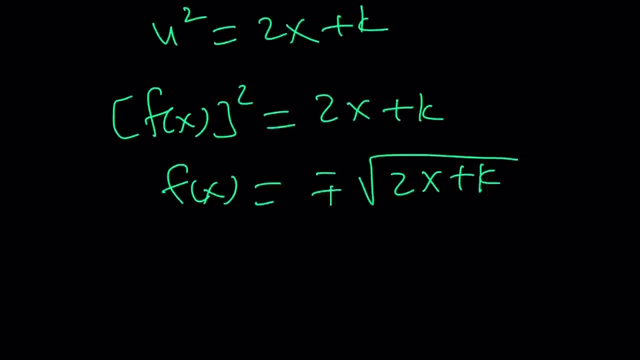 f of x. So we're going to plug it in and then we'll arrive at the exact same solutions as before. So hopefully you're convinced that square root of 2x plus k is going to satisfy. And if you wanted to test it out real quick.